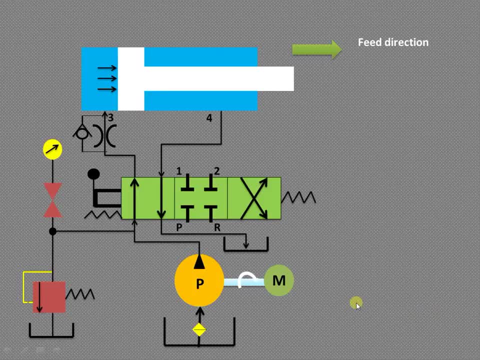 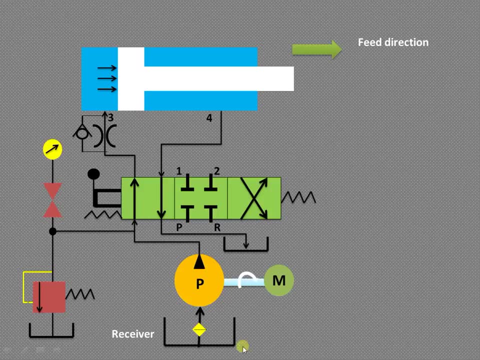 Okay, so let us try to understand how to trace a simple hydraulic circuit As shown over here. we will first try to understand the various components of the hydraulic circuit. So this is the receiver from which the fluid will be pumped by the pump, and the pump is driven by electric motor. This is the strainer which is used to filter that particular fluid. So the pump is fixed displacement pump and it is unidirectional pump. It is rotating in only one direction. 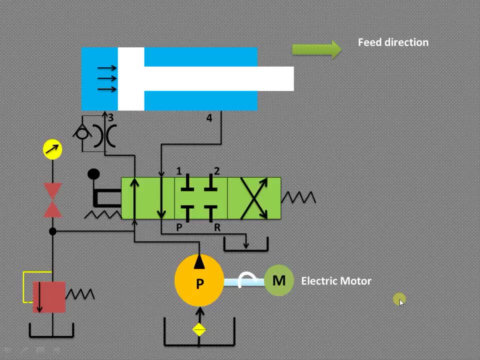 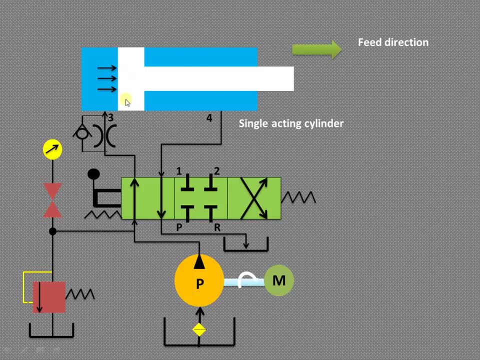 It is driven by the electric motor, as shown over here. The cylinder that we have shown is a single acting cylinder. The fluid is acting only on one side of the piston. The pump pumps the fluid from the receiver and then that particular fluid is sensed by this relief valve. If the pressure is excessive, then the, as compared to the pump, the pump is not acting. 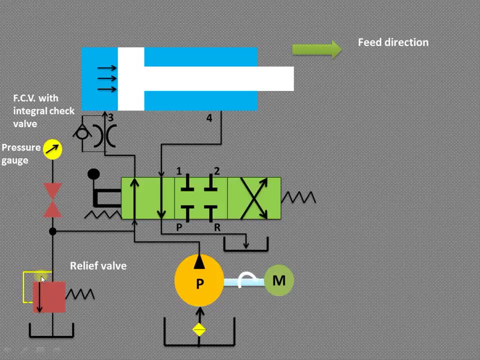 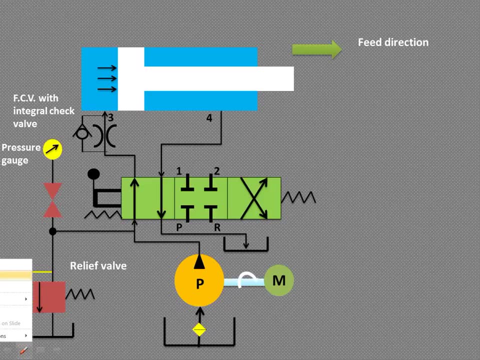 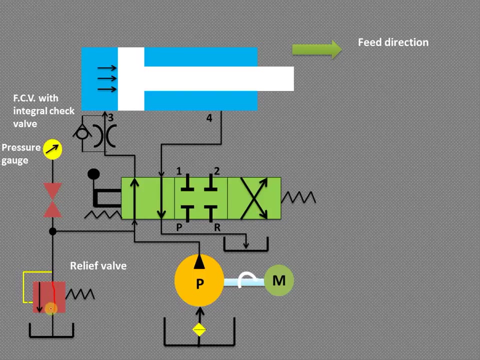 Due to that of the design pressure. generally it is normally close position, as we have shown over here, But if the pressure exceeds a certain design value then it will open and we can say that this arrow that we have shown over here will assume the position in this particular direction. So the position will be like this And again the liquid that will be flowing from this pump over here will be coming over here and then it is going directly again to back to the receiver. So no further operation will be done. 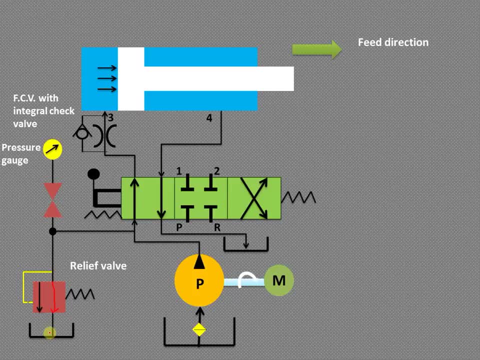 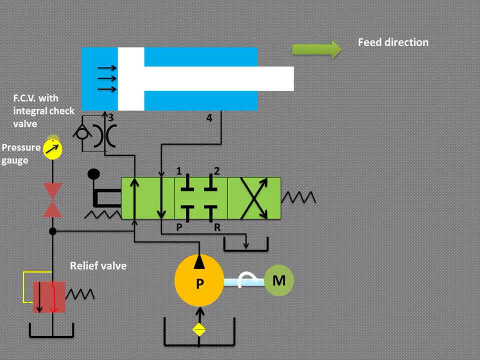 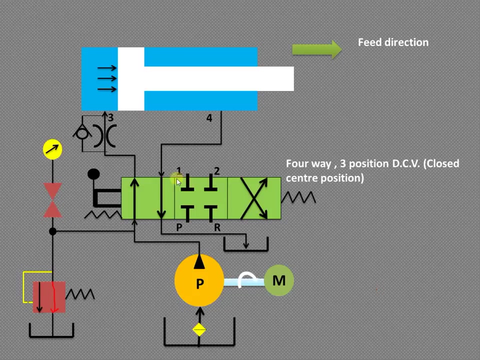 be performed. if the pressure is excessive or if it exceeds the design pressure, Then this is the pressure gauge, which indicates the pressure, and this is the shutoff valve, as shown over here. Now this is the most important part of any hydraulic circuit. So here we have shown. 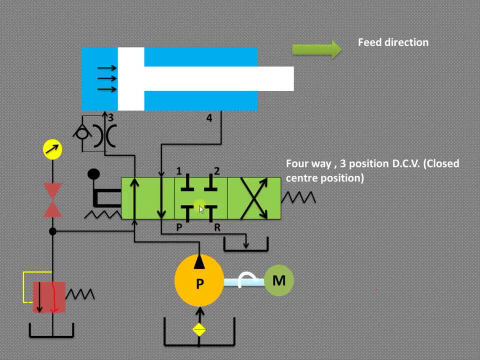 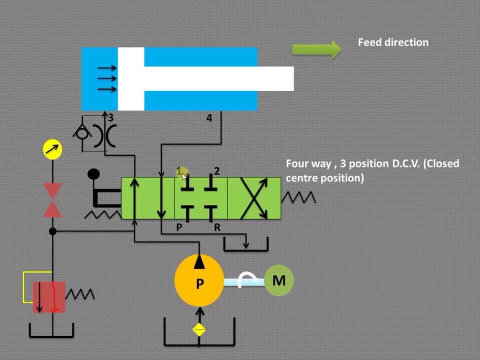 four ways. So these are the four ways: P, R, 1 and 2.. These are the four ways: P stands for the pump port, R for the receiver port, 1, that is the inlet that is given to the cylinder, and 2 will be. 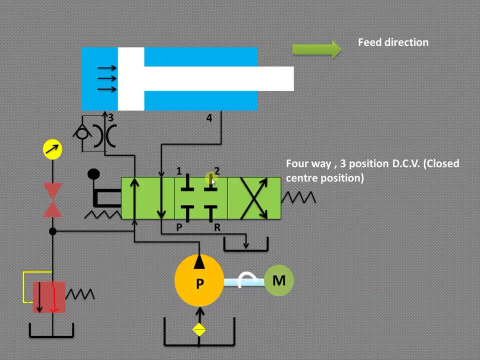 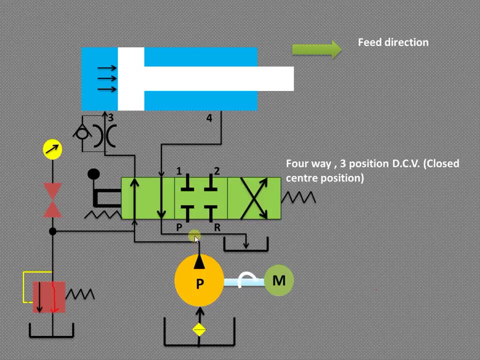 the outlet from the cylinder or vice versa. So here this is the center position and it is the block position. If the fluid comes from the pump and it enters at this particular port P, then nothing will happen. The position of the fluid inside the direction control valve is such that all the ports are blocked and no 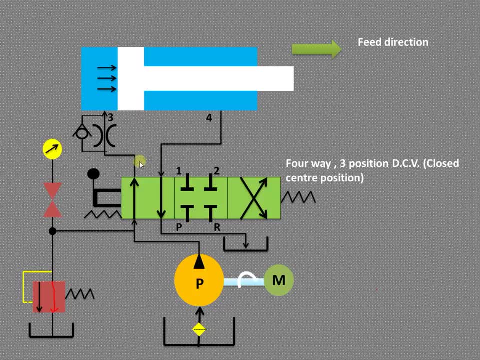 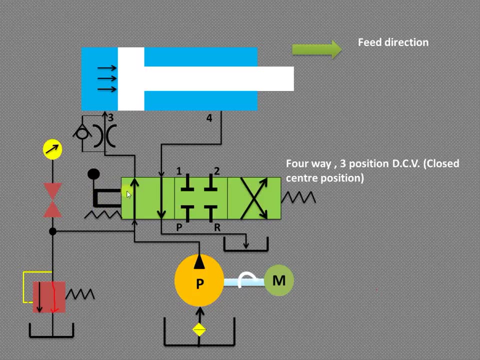 operation will be performed, Rather, no fluid will be given to the cylinder. Now, as we have shown over here, it is a lever operated and spring control direction control valve. So when we operate this particular lever in such a way that suppose we get the left envelope, 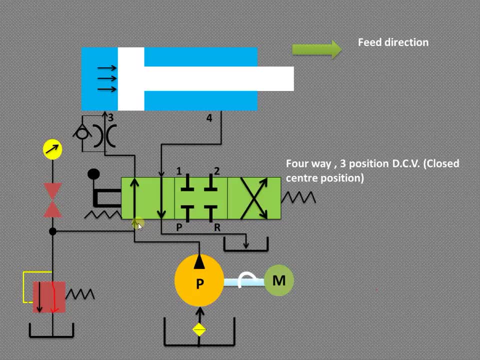 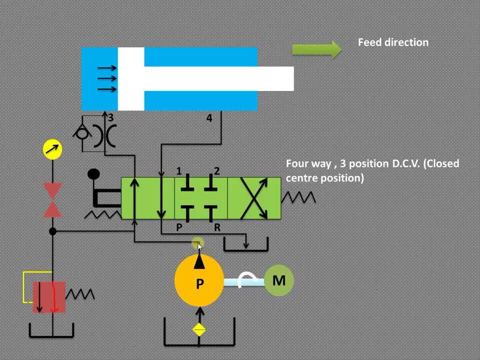 moved, then we can say that P and R will be present over here, P and R Similarly, this 1 and 2 will be present on this particular side and the fluid from the pump will enter this port. P From P it will go to 1 and from this 1 it will enter. 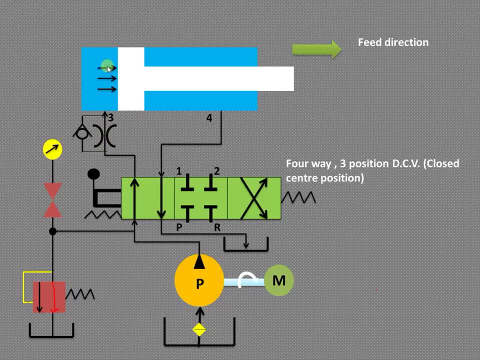 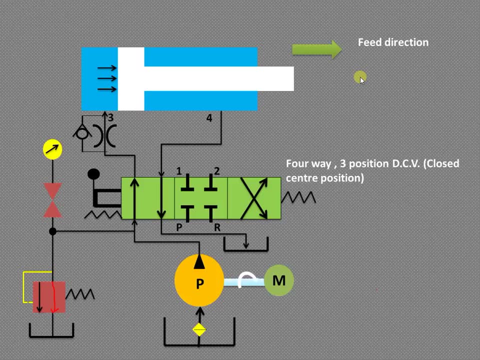 through this restricted opening and it will pressurize this. The force will be acting on this piston and it will cause the piston to move in the forward direction that is known as the feed direction. The liquid from the other side will enter this port 2 and from 2 it will go to R and 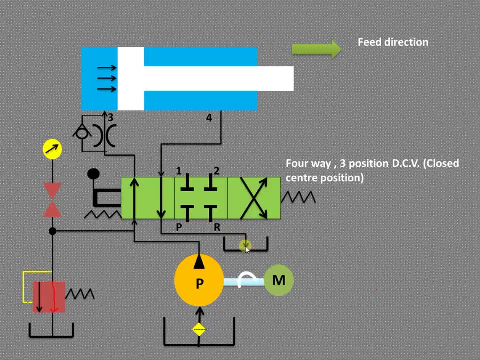 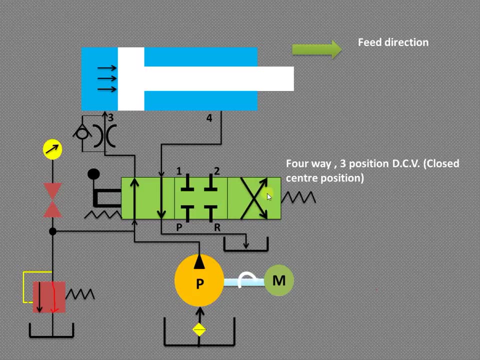 then it will go back to the receiver. When we operate the lever or release the lever in such a way that we get the right envelope moved, then we can assume this particular position that is present over here. So P will be over here. 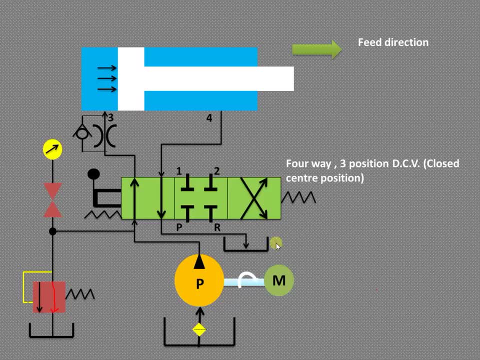 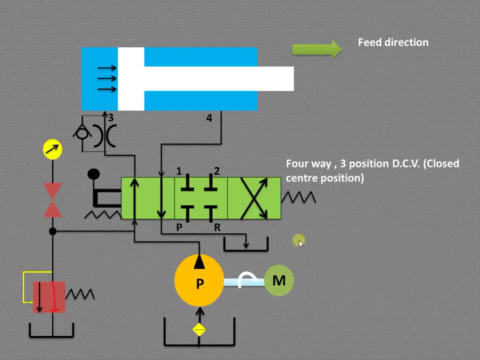 R will be over here, then 1 and 2 will be over here. So the operation of this particular left and right envelope mode will be shown in the next animation. So this is the four-way, three position direction control valve. So these are the four ways: P, R, 1 and 2, and there are three. 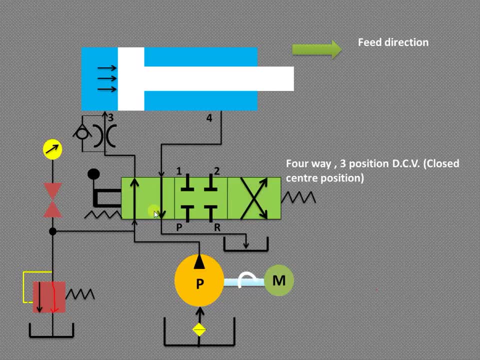 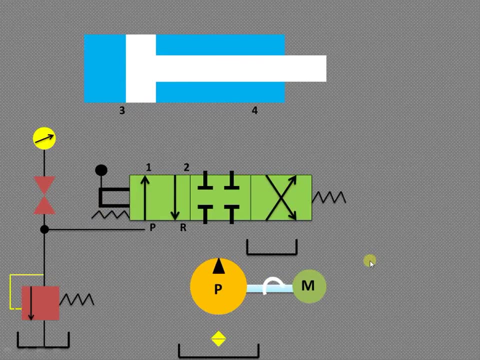 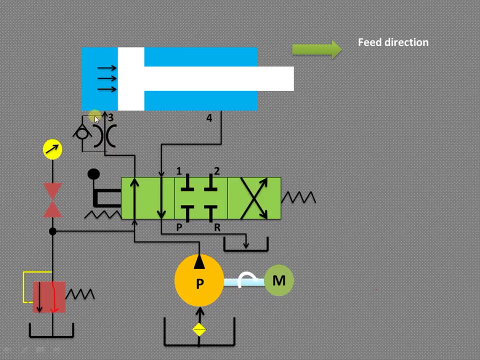 positions, so centre position or close position, and left envelope mode and right envelope mode, and this lever operated spring control. Welcome back to theонother important component. Another important component of the hydraulic circuit is this particular flow control valve with the integral check valve, The check valve. it functions in such a way that it will allow: 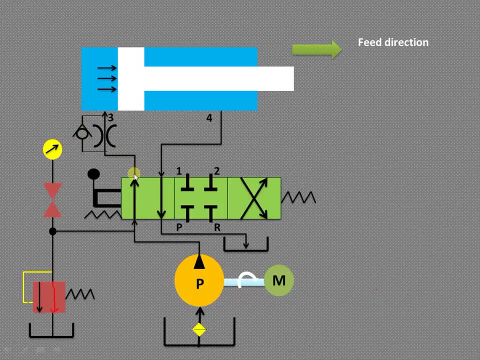 the feed to flow only in one direction. Now, when the fluid comes over here, for example in this particular position, then the flow kunitama will go below The flow kunitama will be moving in this particular position and it will push the financial flow guy over the Drum Juck. Now, when theark. 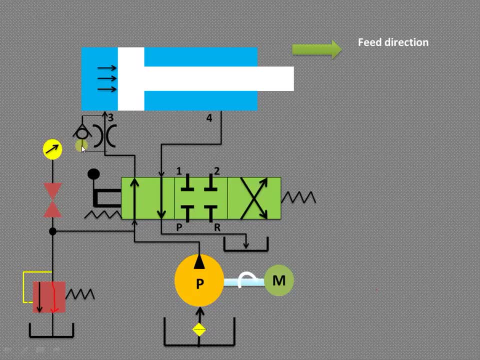 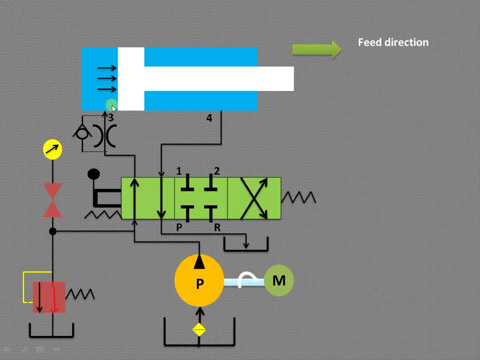 will come over the благодар physical flow qu0ts point. then it will move to the coming current from the. it is a no free flow condition or no flow condition for the check wall, so liquid cannot flow in this direction. so it has to compulsorily flow through this restricted opening and then. 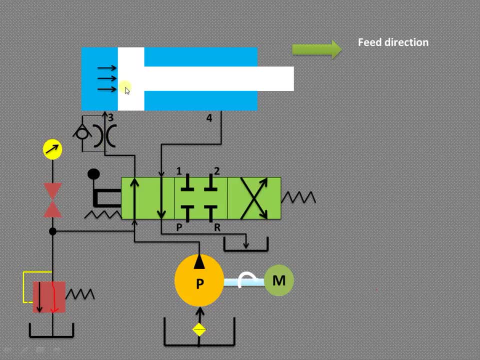 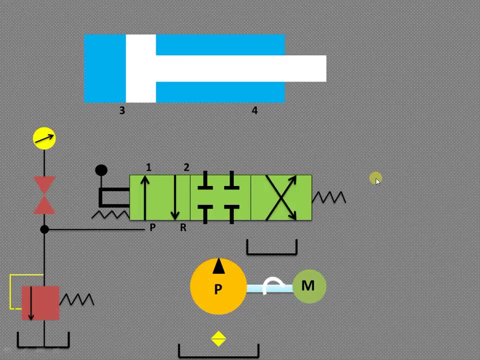 enters on this particular in cylinder end of the, this particular single cylinder. now let us try to understand this: the forward motion of the piston through this animation. so liquid from the reset reservoir or receiver it is pumped by the pump. okay, then it will enter to this port p. from port p it goes to port one, from one it will enter to the port three and it 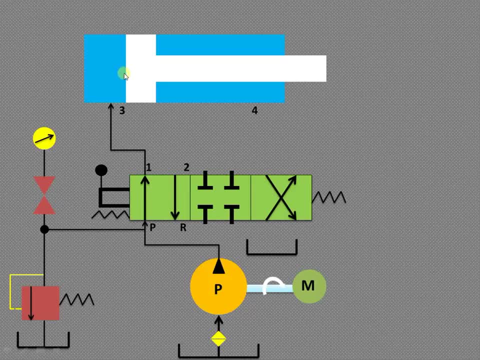 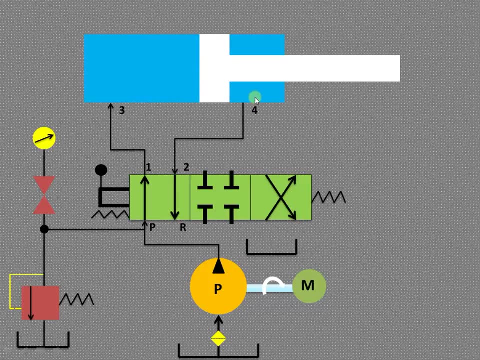 the fluid will be allowed to act on this surface of the piston so that it will move in the forward direction. the liquid from the other end, that is the rod end, will enter from four to two and from two it will go to the reservoir. so from two to r. so in this way you can trace. 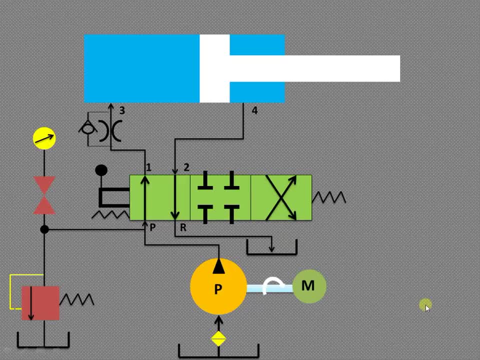 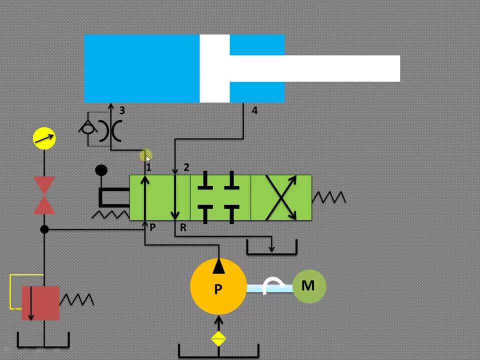 this particular hydraulic circuit. so here now we'll try to understand how this particular flow control valve works. so here the liquid will come over, here it cannot go from this side. it is because this is a no flow condition, but it has to come. it has to flow through this restricted 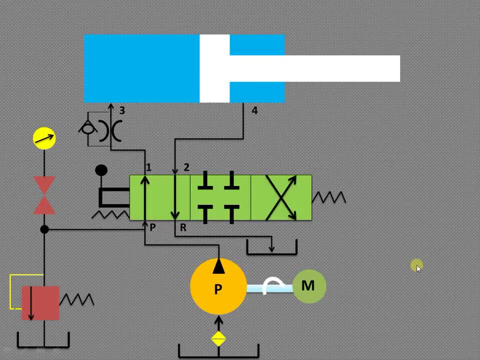 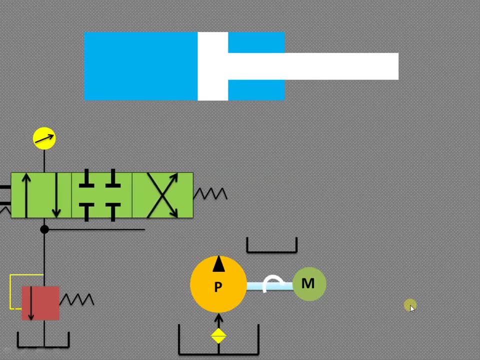 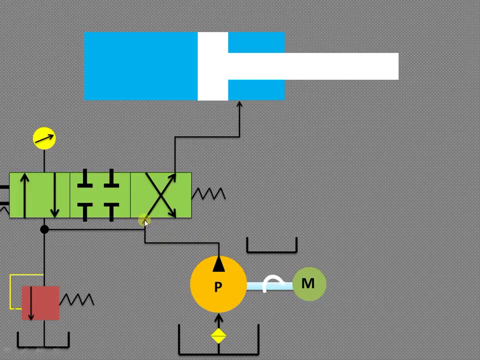 opening. so piston will move slowly in the forward direction. so this is our left envelope mode. now will see the right envelope move. so let us animate in such a way that you can easily understand this particular concept. so now from the pump the liquid is allowed to enter over here from this side. it will go to this port from this. 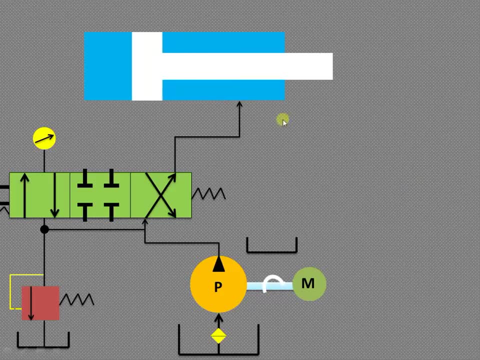 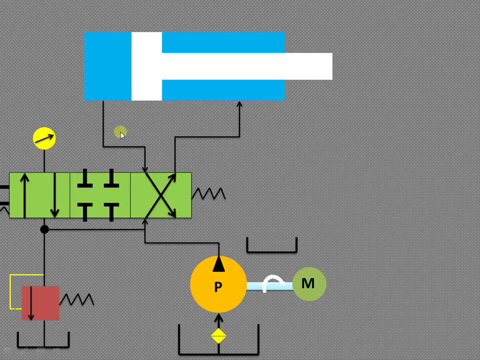 to this rod end of the cylinder will cause this piston and piston rod arrangement to move in the backward direction. the fluid from the other side will enter over here and from this it will go to the reservoir. but now you can see, it can easily flow through this check wall because this is a free 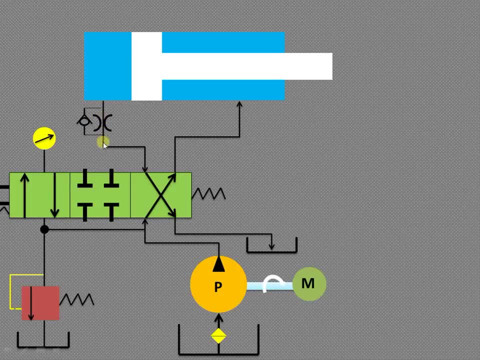 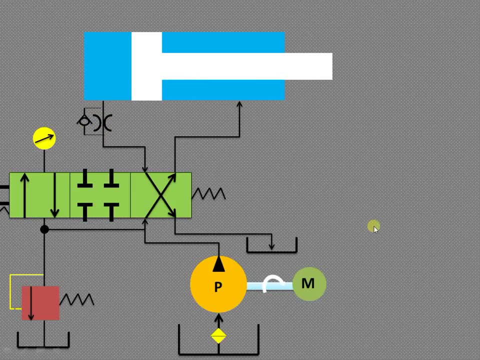 flow condition of the check wall as well, as it can flow through this restricted opening also correct. so the backward motion will be fast because there is no restriction to the flow of the fluid from this port to the, from this port 3 to the port 1 and from 1 to R and then to the reservoir.